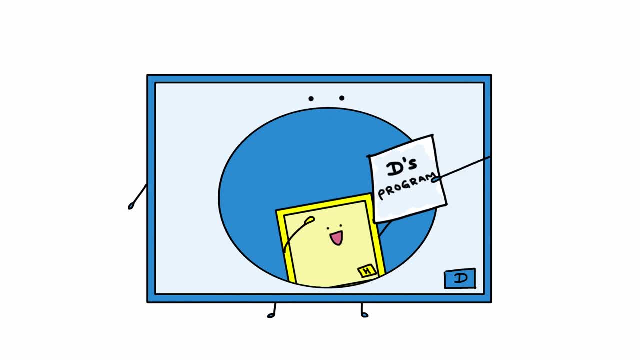 So when D takes in its own program as input, it passes it to H and H decides whether D will halt. Let's say H determines that D will halt, but because D is designed to do the opposite of what H says, then D ends up running forever, even though H said D will halt. 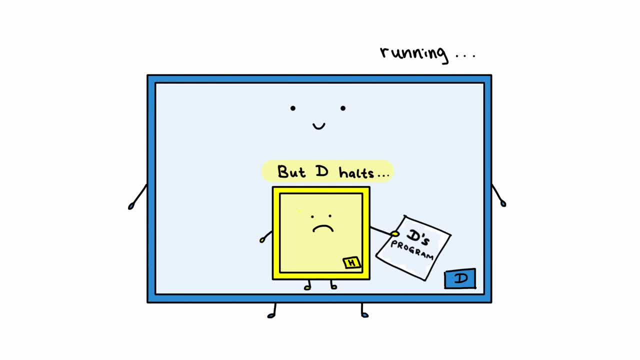 This means H is wrong, But we assumed in the beginning that H is always right. So let's try again. D takes in its own program and passes it to H, but this time H says D does not halt and runs forever. And again, because D is designed to. 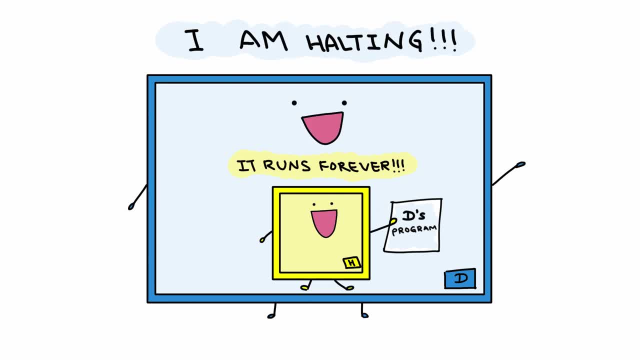 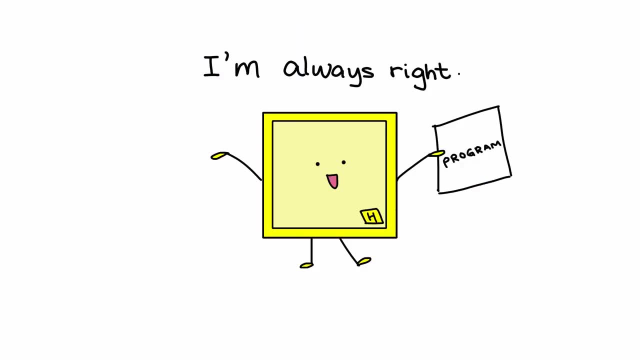 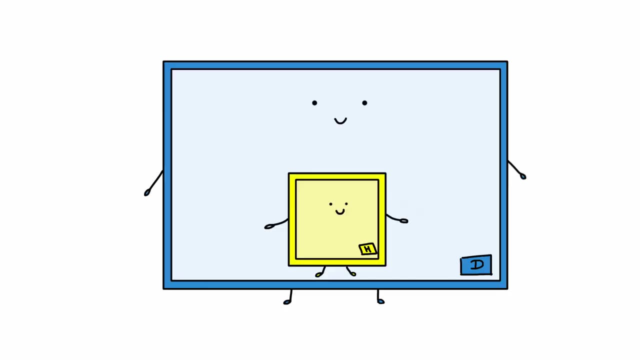 do the opposite of what H says. D halts. H is wrong again. But remember, in the beginning we assumed that this magical program H always correctly tells us if a program will halt- exists. But our experiment with D just showed that if H existed and we built D using H, then H can be. 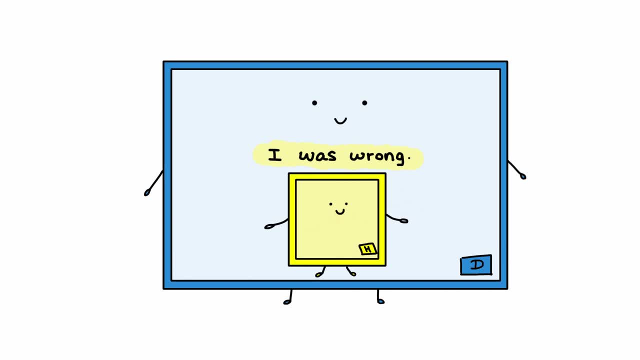 wrong. This contradicts our initial assumption that H is always right. Therefore, a program such as H that correctly determines if another program will halt cannot exist. Therefore, a program such as H that correctly determines if another program will halt cannot exist. 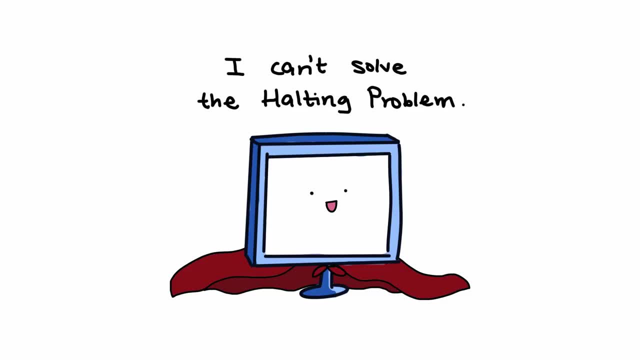 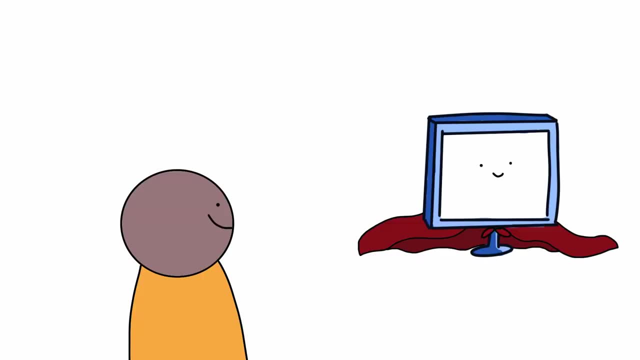 So that's the halting problem. And again, not even the most powerful supercomputer will be able to solve the halting problem. Asking a supercomputer to solve the problem would be like asking the supercomputer to come up with a triangle with four sides. 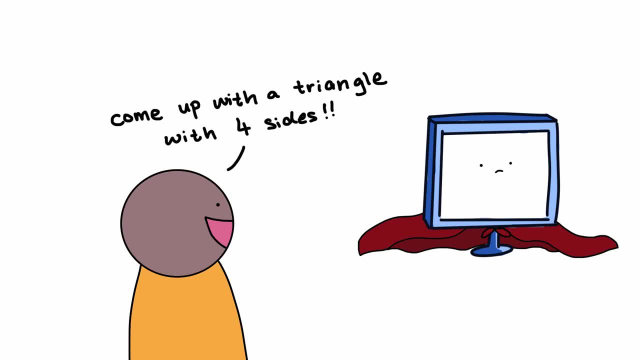 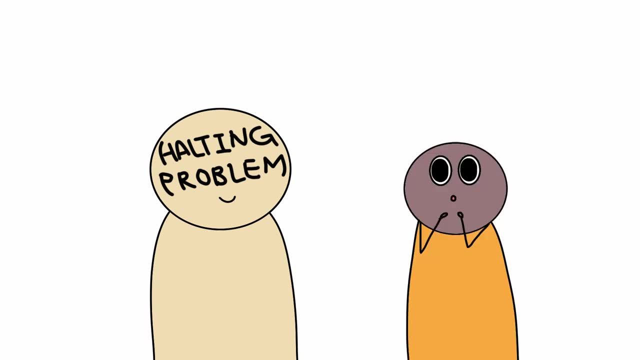 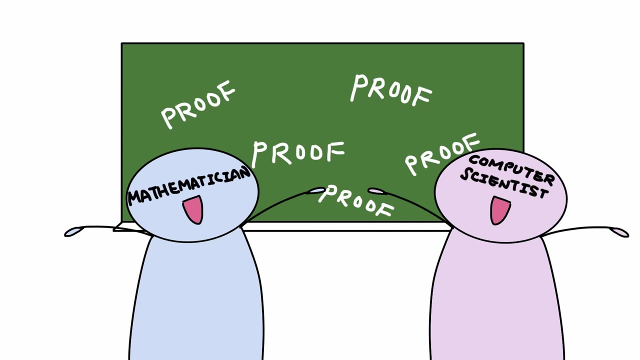 Logically, it makes no sense. So yeah, the halting problem is pretty significant and mind-blowing when you really think about it. It's also just incredible how mathematicians and computer scientists have rigorously proved that there are problems that can never be. 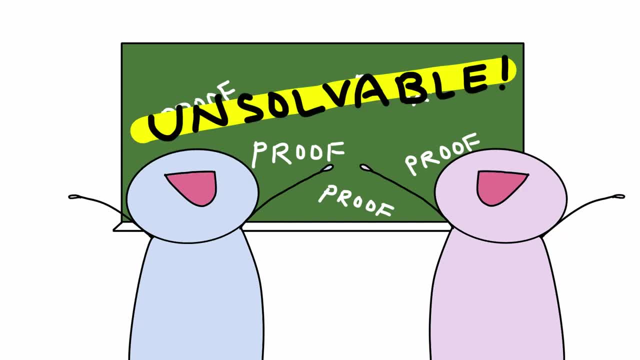 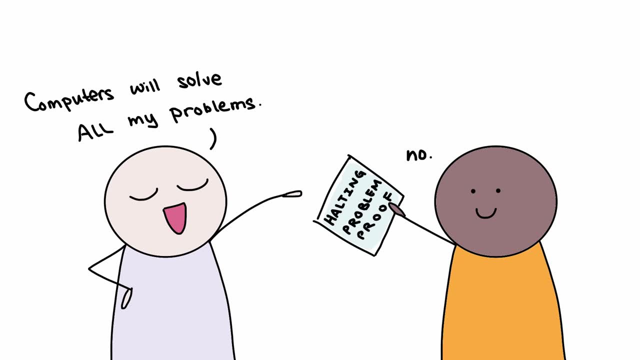 algorithmically solved. So the next time someone tells you that computers will one day solve everything, just tell them about the halting problem.